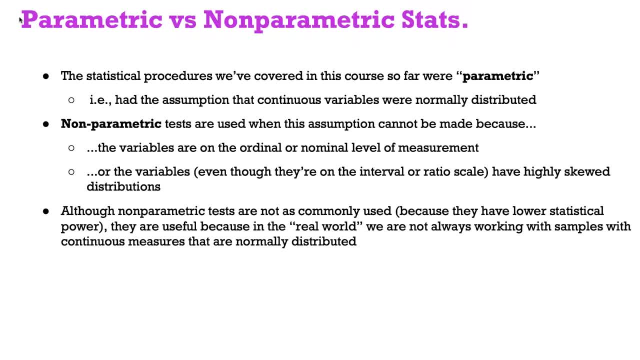 distributed. Non-parametric tests, on the other hand, are used when this assumption cannot be made, because either the variables are not continuous, ie either ordinal or nominal, or the variables are highly skewed, even if they are continuous. So non-parametric tests. 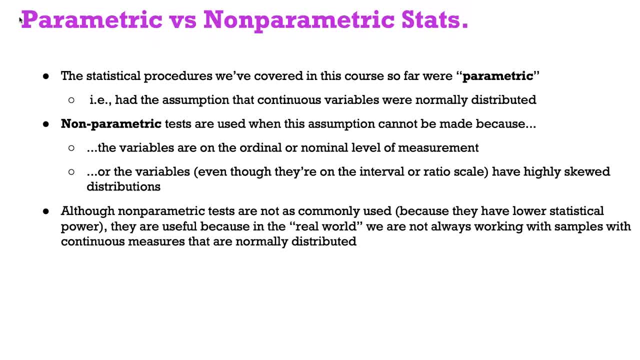 they're not as commonly used because they have lower statistical power, but they're useful in real-world settings. We don't always have samples that have variables that are measured on a ratio or interval scales, or even if they are, they might not be normally distributed, And so we 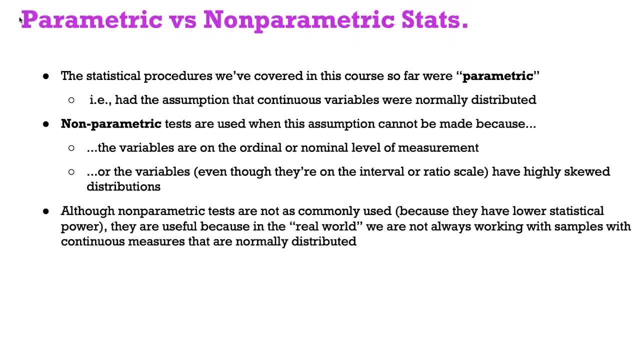 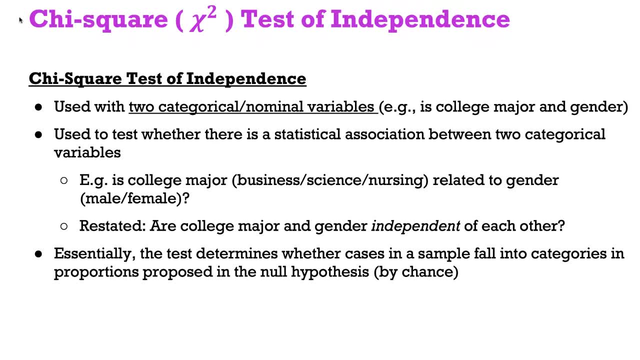 could use non-parametric tests to determine if they're useful or not. So, for example, is significance. So the chi-squared test of independence is used when there's two categorical or nominal variables, ie college major and gender, and it's used to test whether. 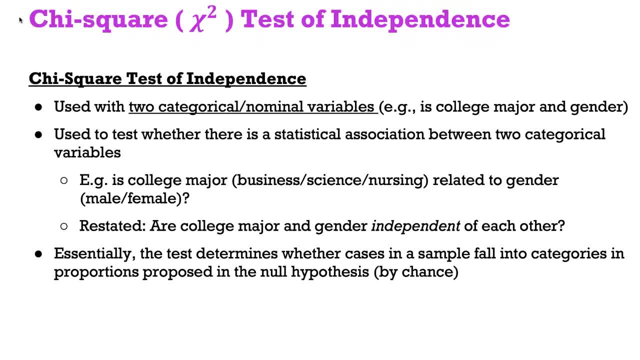 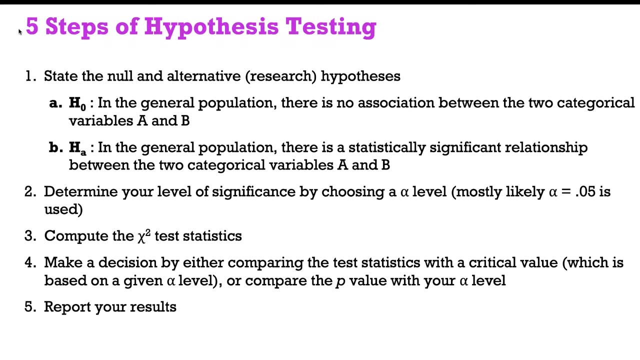 there is a statistical association between these two categorical variables. So are college major and gender independent of each other or does one impact the other? Essentially, this test determines whether cases in a sample fall into categories in proportions proposed to the null hypothesis or by chance. So we again use the five-step hypothesis to test this. 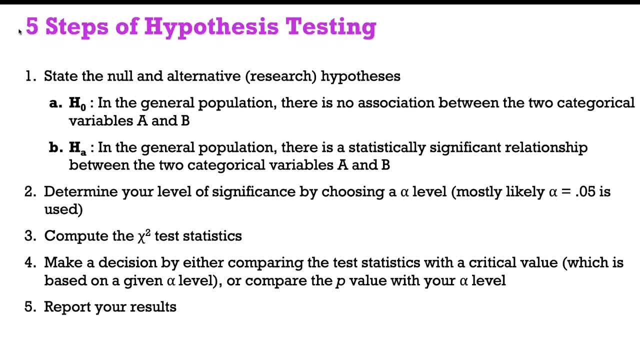 We state our null. and our alternative, Our null hypothesis, is that in the general population there's no association between the two categorical variables A and B. Alternatively, there is a statistically significant relationship in the general population between the two categorical variables A and B. We set our alpha at 0.05.. 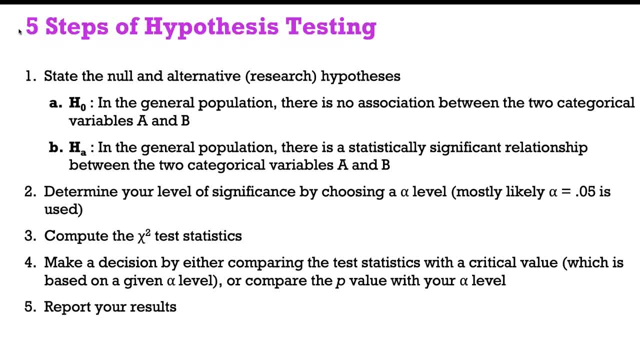 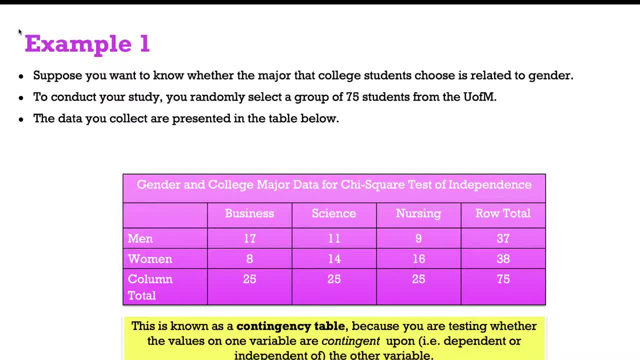 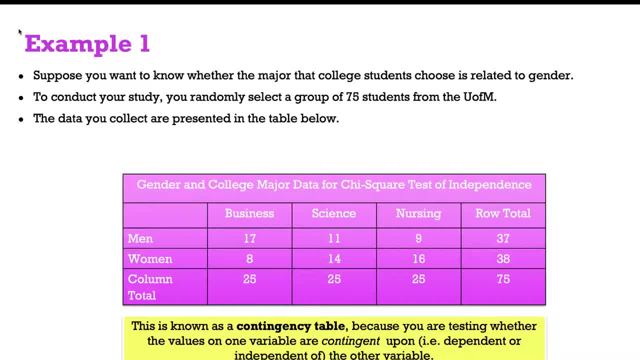 choose is related to their gender. So we conduct our study. We randomly select 75 students from the University of Memphis and this is the data that we've got. So we can see that there are 25 business majors, 25 science majors and 25 nursing majors. In business, there's 17 men and 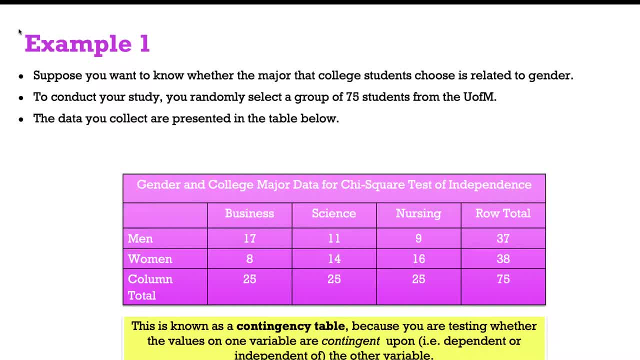 8 women. In science, there's 11 men and 14 women. In nursing, there's 9 men and 16 women. Down at the end we can see that we have a total of 37 men and 38 women in our sample. 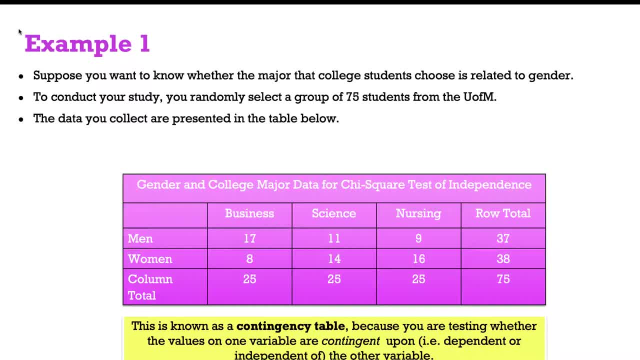 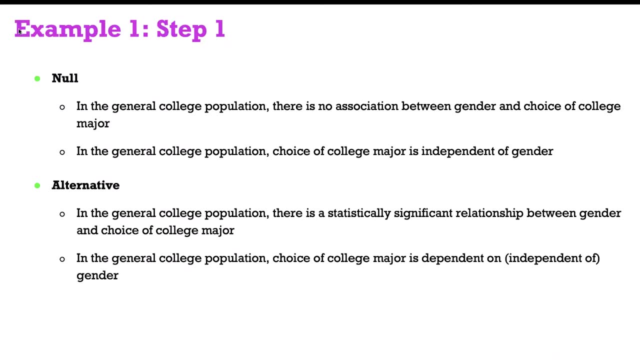 and we have 25 of each of the majors. This table is called a contingency table and it is what we are going to test compared to what we would expect if gender and major were not associated at all. So null hypothesis. In the general college population there is no association between gender and choice. 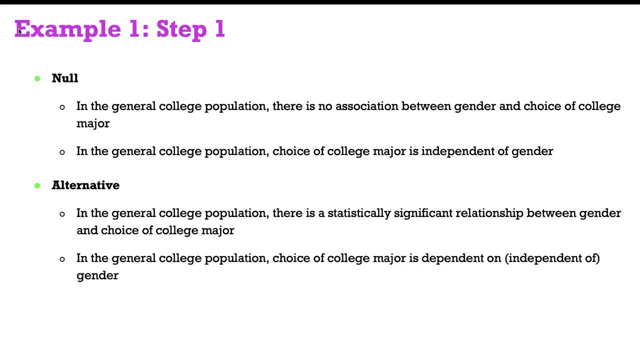 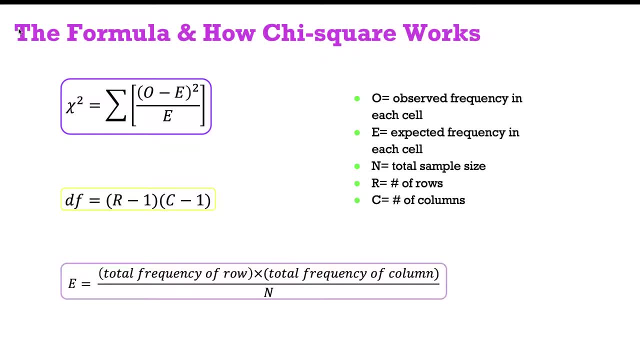 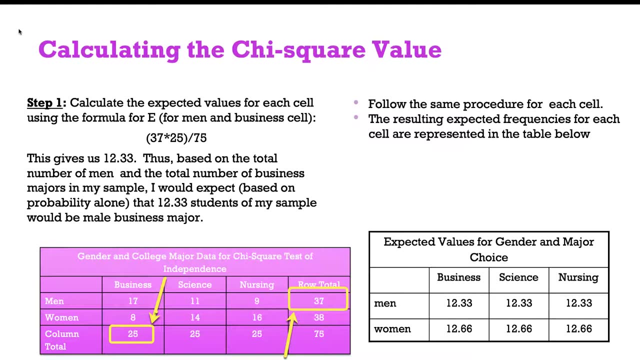 of college major. Alternatively, in the general college population, choice of college major is dependent upon gender. There is a formula that you can use to calculate this and essentially what we're doing is we're comparing our actual values in the pink, what we found with the expected values. 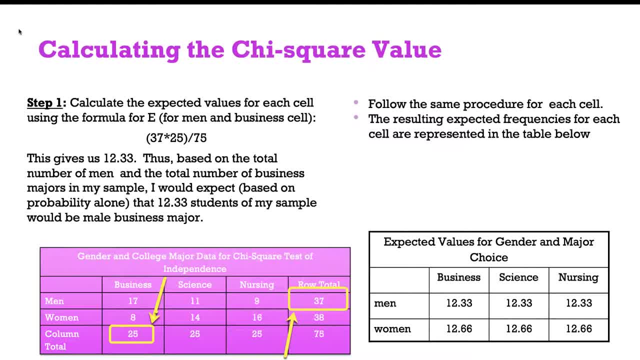 if they're not associated with gender. So we're going to test that. So we're going to test that. So there was no association between gender and college major. So if there's no association between what your gender is and what major you select, we would normally expect, given our population. 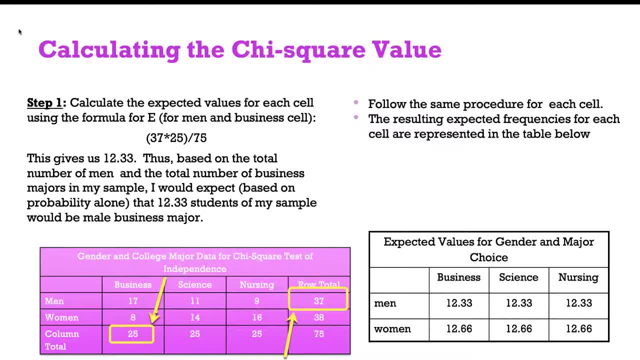 given a sample of 75 students to find 12 and a third men selecting business, 12.33 selecting science and 12.33 selecting nursing, And if there's no association between gender and college major, we'd expect 12.66 women to fall into business, science and nursing and we'd expect 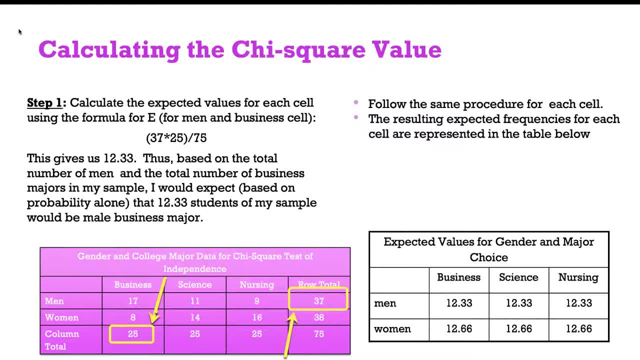 them to fall into business, science and nursing. So if there's no association between gender and career, we're not going to try to ПП our example of does 3 equal 3 intuitions and does an skinny 16 say Ron two senate doesn't make the spoiling of um can remember meaning. However, if there's means for 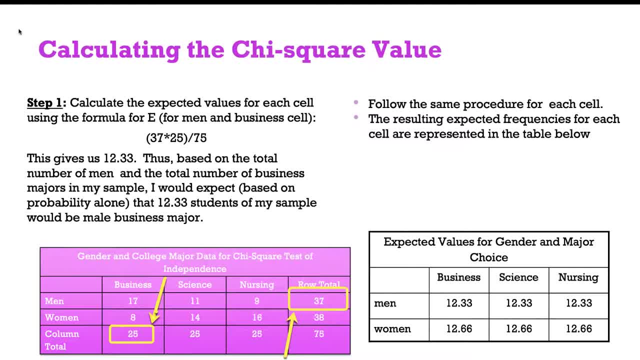 it. we're still going to tryERA conclude that it's freaking natural that there's no association and nursing equally. However, this is not the case. right, We can see that we had 17 men in business, 11 in science and 9 in nursing. So what we want to do is we want to know: is there? 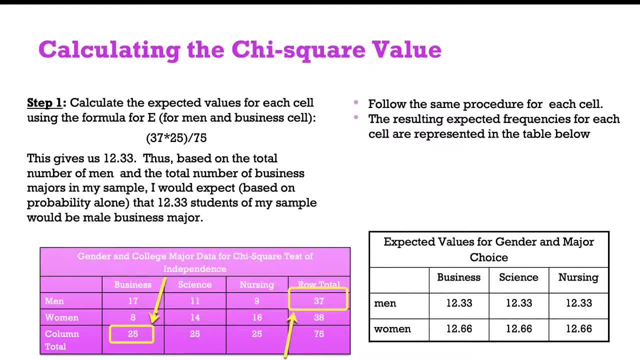 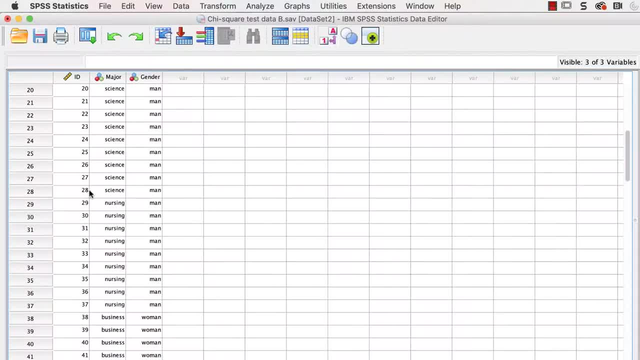 a significant relationship between gender and college major. So we will go into SPSS and test this. So in SPSS we can see that we have our participant ID and we have 75 participants. We have the three majors- nursing, science and business- and the two genders, for man and woman. 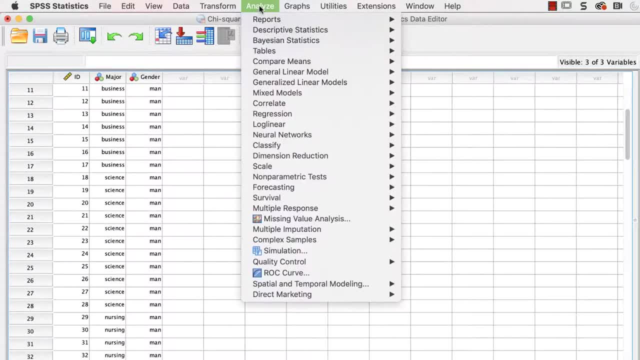 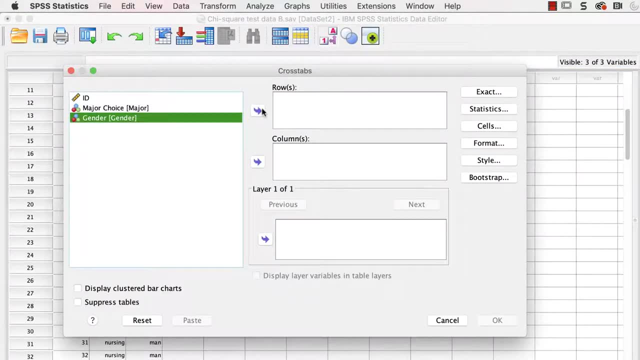 So what we'll do in order to run our chi-squared is we'll go to analyze descriptive statistics, cross tab, We'll move our gender into our rows and major choice into the column, Just like we had in our contingency table. We want to click statistics and then chi-squared. 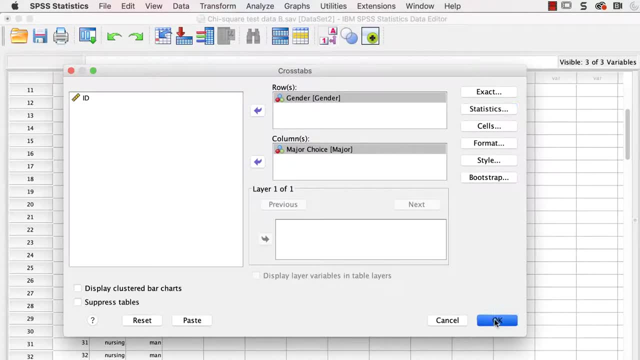 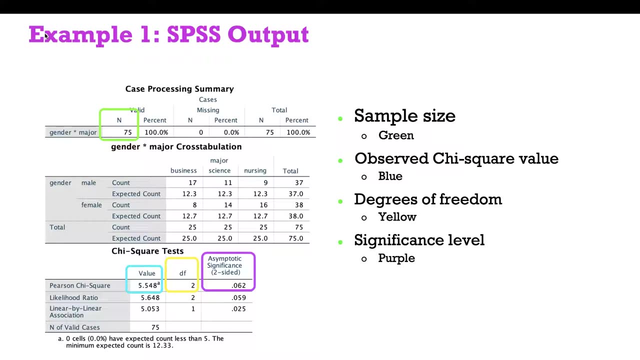 and hit OK And then click OK. In our output we get three tables: our case processing summary, which is our descriptive statistics, And this is going to tell us our sample size, which was 75.. The next thing we get was the gender times major cross tabulation. This is essentially 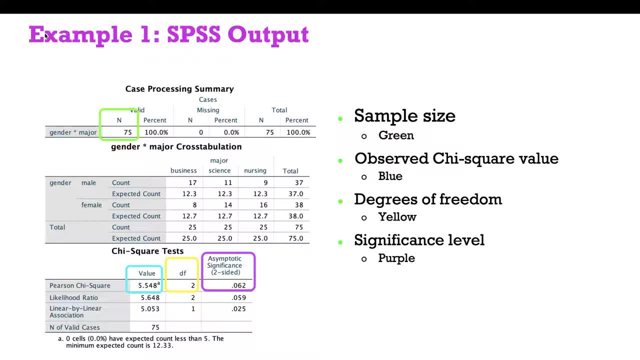 our contingency table that was in pink before, And then we get our chi-squared- and this is going to be what we're looking at- to determine if we have a significant association between the two categorical variables. So we can see in the Pearson's chi-square that our 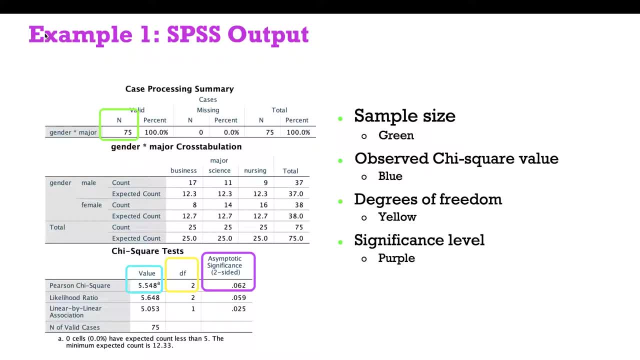 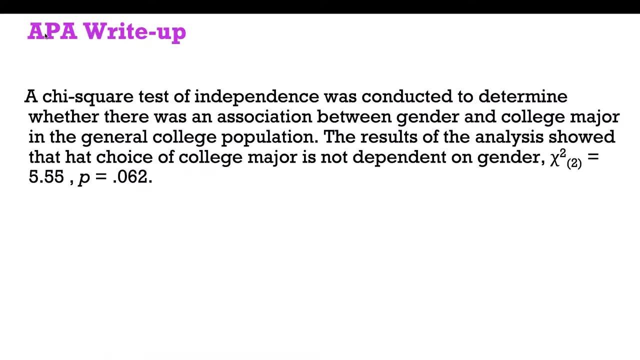 chi-square value is 5.548 or 5.55, if you round with two degrees of freedom and a p-value of 0.062.. So we'll write this up. A chi-squared test of independence was conducted to determine whether 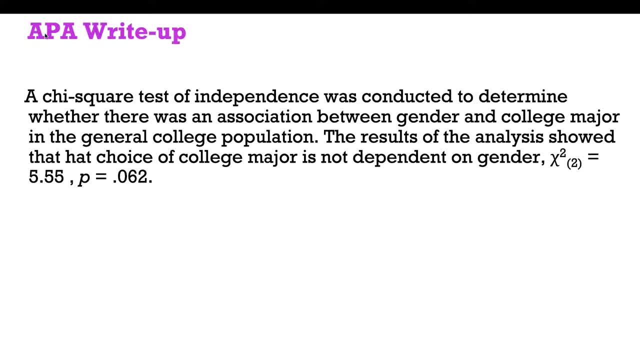 there was an association between the two categories, So we'll write this up. A chi-squared test of independence was conducted to determine whether there was an association between gender and college major in the general college population. The results of the analysis showed that choice of 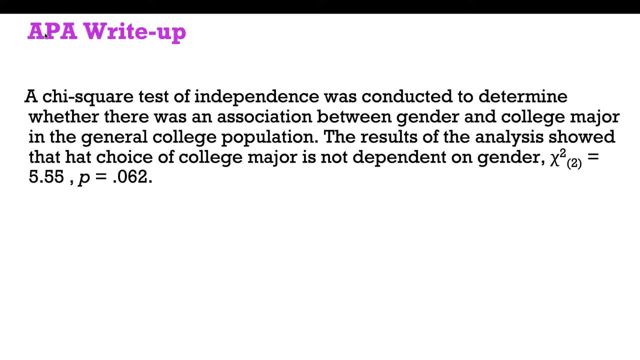 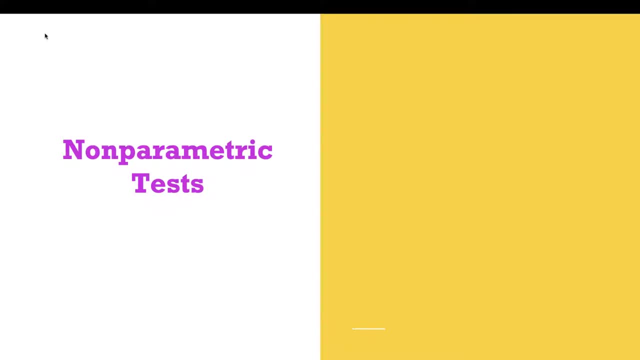 college major is not dependent on gender. There's no significant relationship. Chi-squared parentheses two- for degrees of freedom equals 5.55,. p equals 0.062.. We have some other non-parametric tests that are commonly used. The first is the Mann-Whitney U-test. 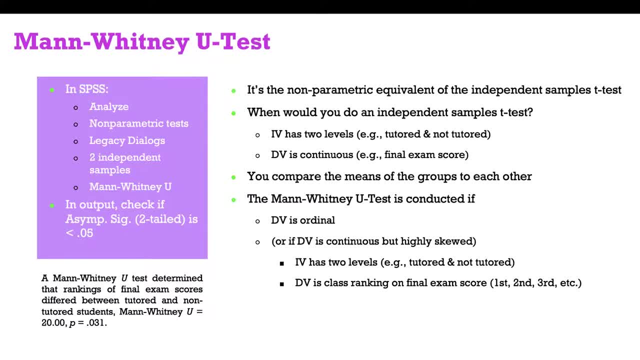 In all of these slides there is a purple box that will tell you how to do this in SPSS. However, you do not have to do this. The Mann-Whitney U-test is the equivalent of the independent samples t-test or two sample t-test, So we would use an independent sample t-test when our 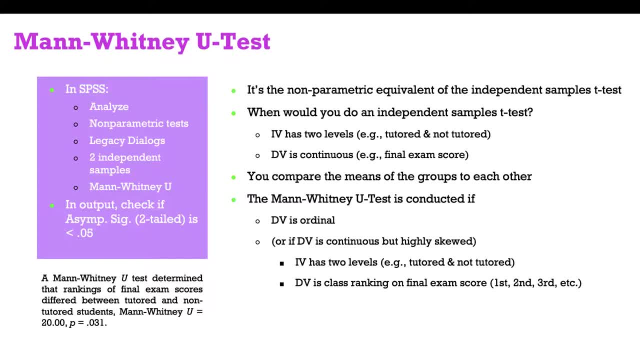 independent variable has two levels- tutored or not tutored- and the dependent variable is continuous, like final exam score, 0 to 100.. We're essentially comparing the means of the groups to each other. The Mann-Whitney U-test, our non-parametric version, is conducted if 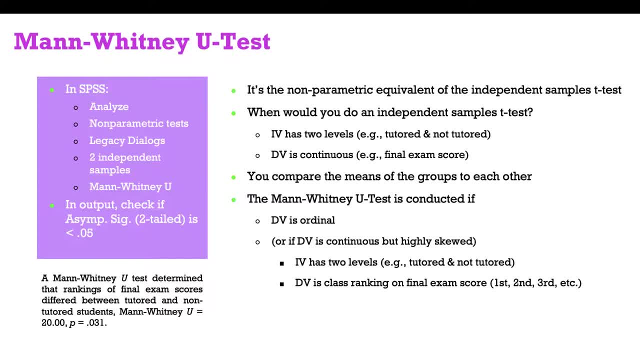 the dependent variable is ordinal, So you know if it is first, second, third, fourth, fifth. So we have our independent variable, two levels- tutored or not tutored- and our dependent variable is class ranking based on your final exam. So first place.